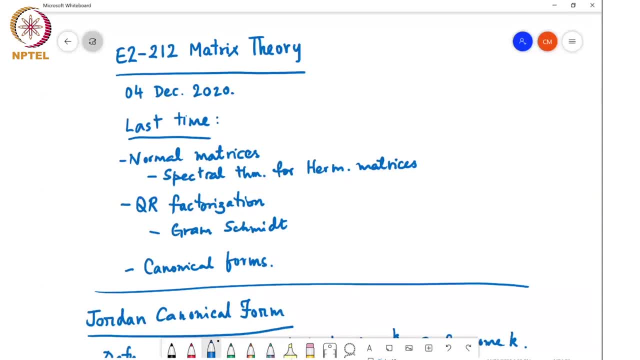 canonical forms. Canonical forms are a way to reduce a matrix to a simpler form, which will allow you to compare matrices and see whether they have the same canonical form or not, which in turn allows you to conclude whether those matrices are going to be similar. 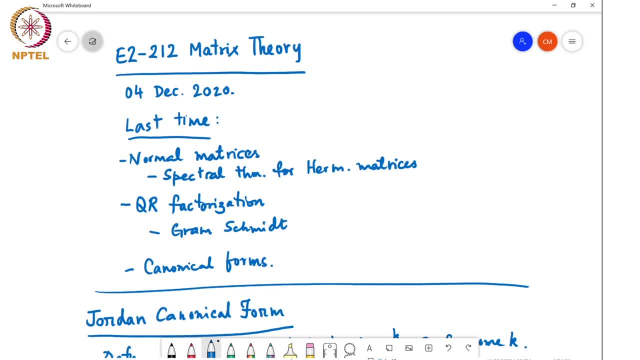 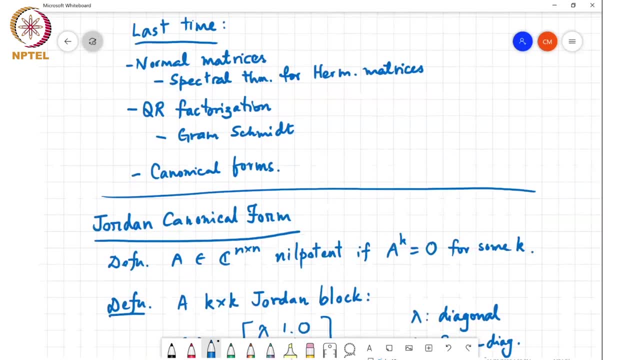 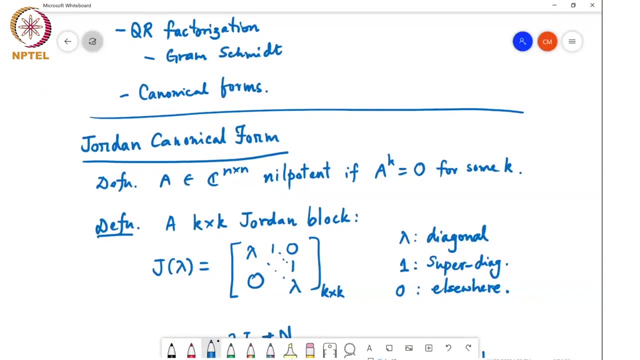 or not, And there are many other uses which we will discuss in the course of these lectures. Now, the specific form that we started discussing is what is called the Jordan canonical form. So, just to recall, a matrix A is said to be nilpotent of order k or index k. 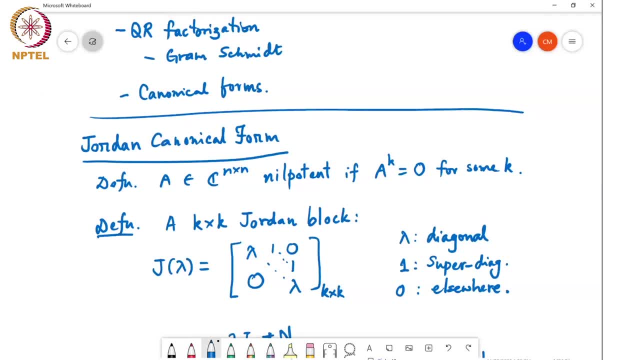 if a power, k equals zero for some value of k And typically the index, what we call the index- is the smallest dimension or the smallest power you need to raise it to so that you get the zero matrix. So, for example, if I take the 2 cross 2 matrix, 0, 1, 0, 0, this is nilpotent of index 2,. 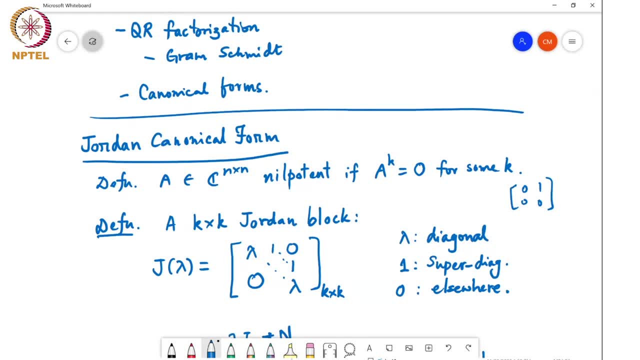 because when I take the square of this matrix I get the all-zero matrix. So basically the Jordan canonical form theorem will say that every matrix is similar to a matrix of the form d plus n, where d is a diagonal matrix and n is 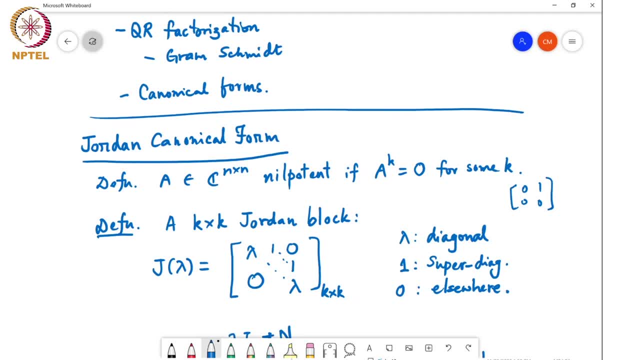 an nilpotent matrix. So one other definition is that of a Jordan block. A Jordan block j of lambda is of size some k cross k, where basically you have lambdas on the diagonal, ones on the first super diagonal, and zeros everywhere else in the matrix. 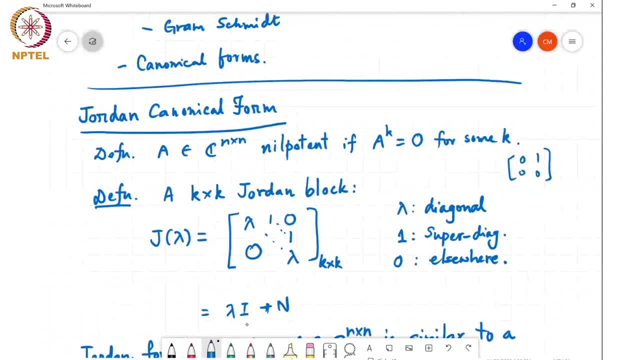 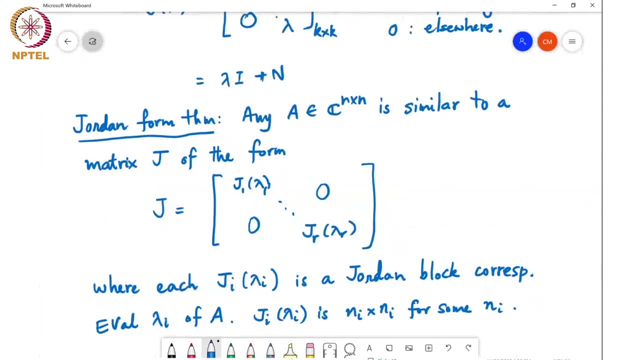 This. you can see that this is of the form lambda times. the identity matrix of size k cross k plus an nilpotent matrix because it has only ones on the first super diagonal. So the Jordan form theorem basically says that any matrix A of size n cross n is similar to a. 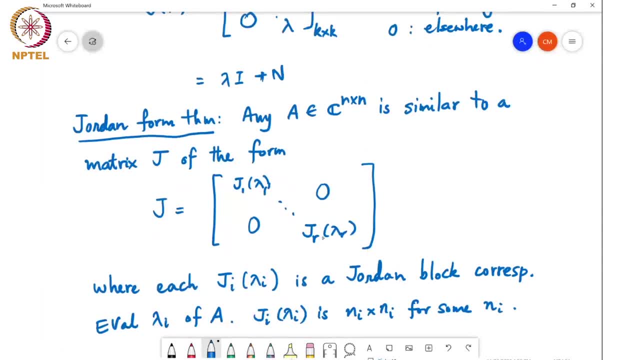 matrix J of this form. So it's a block diagonal matrix with Jordan blocks along the diagonal and there are such Jordan blocks And each J of this form is a block diagonal matrix and the J of lambda is a block diagonal matrix. So this is a Jordan block corresponding to. 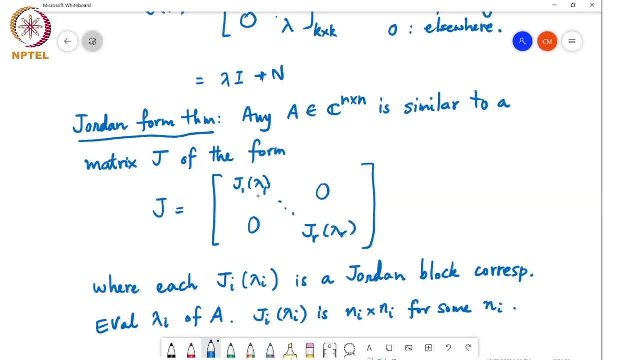 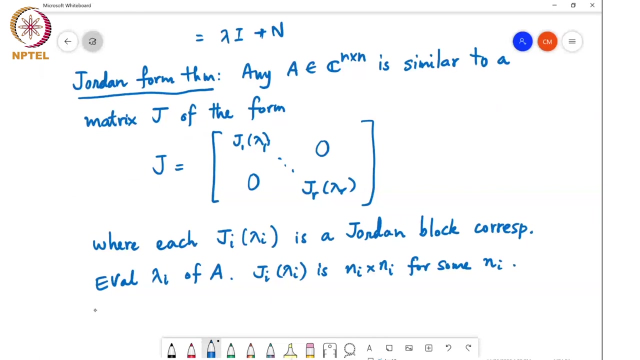 eigenvalue lambda i of A, So the same value of the same eigenvalue could be repeated in multiple blocks. This block is of size n. i cross n i for some value of n i, So, for example, n i could even be equal to 1.. Okay, So just to clarify what this theorem is saying, here are a few. 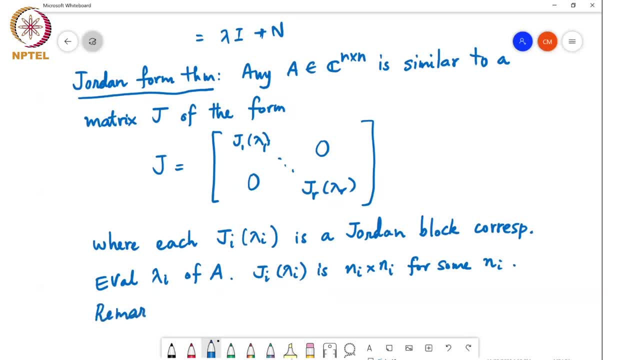 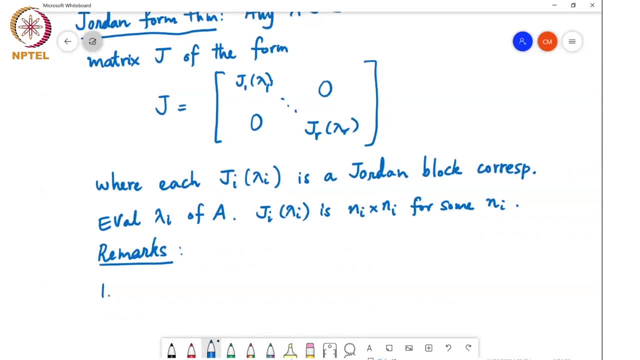 marks. First, these lambda i's need not be distinct. That is the same lambda. i could occur in multiple blocks. So this is the same lambda. i could occur in multiple blocks. So this is the same lambda. i could occur in multiple blocks. The second is that this decomposition into this 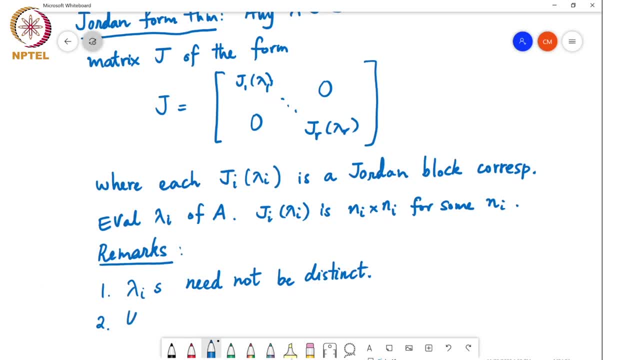 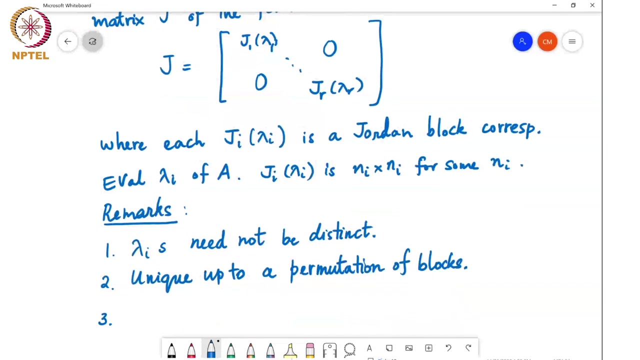 canonical form is unique up to a permutation of blocks. And third point, this matrix J is called the Jordan canonical form of a. Thank you very much for yourão. Thank you very much for yourão. Thank you, Thank you very much. 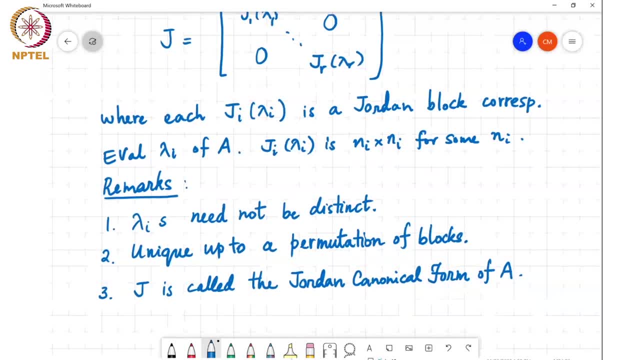 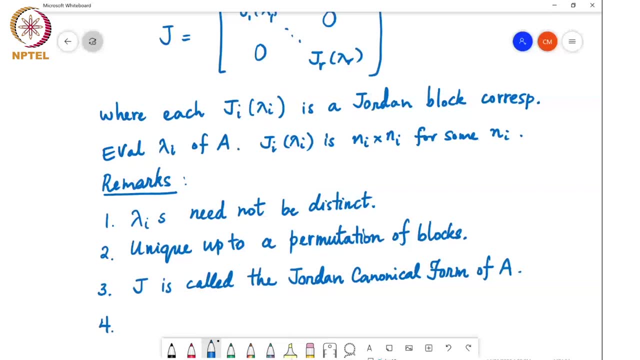 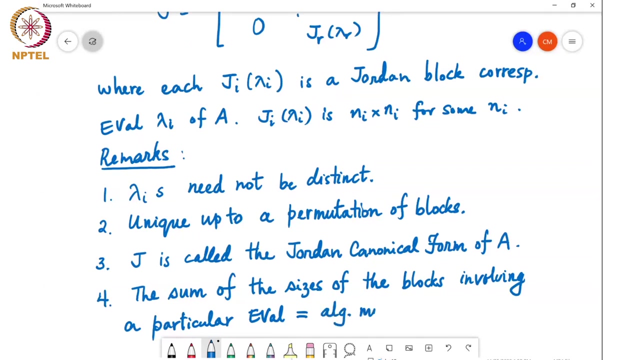 Thank you very much. Thank you. So the sum of the sizes of the blocks involving a particular eigenvalue is the algebraic multiplicity of that eigenvalue. So what is the algebraic multiplicity? So what is the algebraic multiplicity? 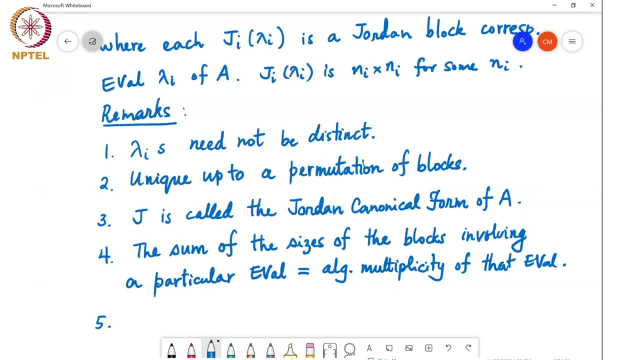 So what is the algebraic multiplicity? It is the number of times that the particular eigenvalue occurs as root of the canonical triangle. So basically, the Jordan canonical form will reveal the algebraic multiplicity of all the eigenvalues of the matrix. 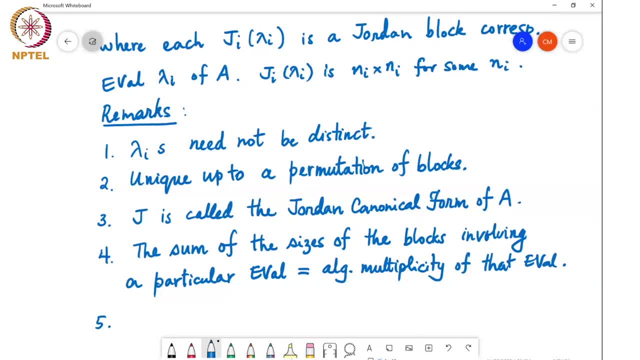 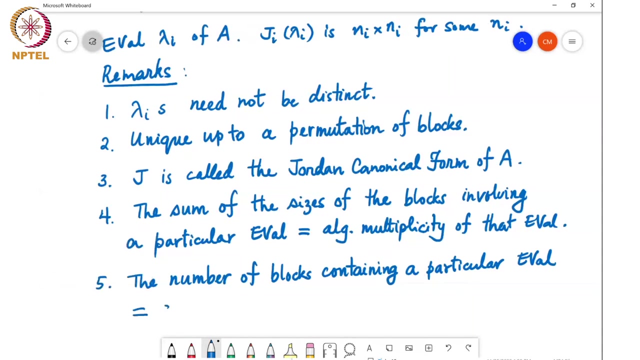 Or it contains in it the information about what the algebraic multiplicity of every eigenvalue of the matrix is. The number of blocks involving a particular Eigen value is the geometric multiplicity of that Eigen value. So what is the geometric multiplicity? 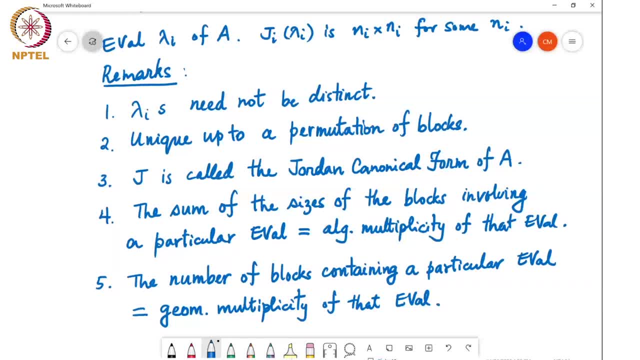 It is the dimension of the Eigen space corresponding to that Eigen value, or in other words, the number of blocks involving a particular Eigen value. So what is the geometric multiplicity? It is the dimension of the Eigen space corresponding to that Eigen value, or in other words, the 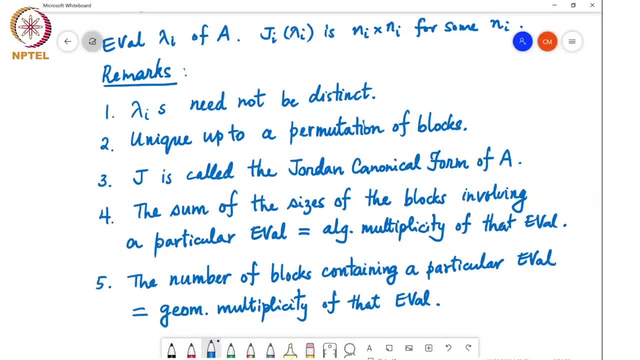 number of linearly independent vectors, or linearly independent Eigen vectors that you can find corresponding to that Eigen value. That is the geometric multiplicity and that equals the number of blocks containing a particular Eigen value. So if the algebraic multiplicity is equal to the geometric multiplicity for every Eigen, 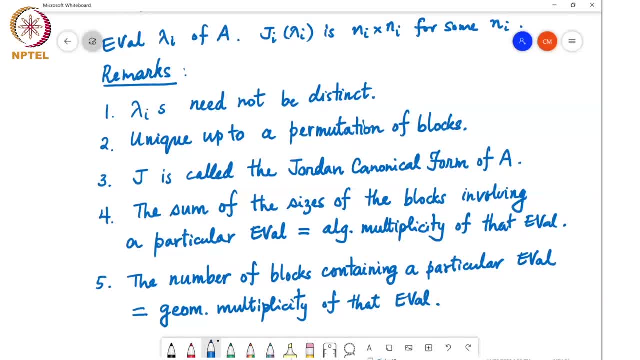 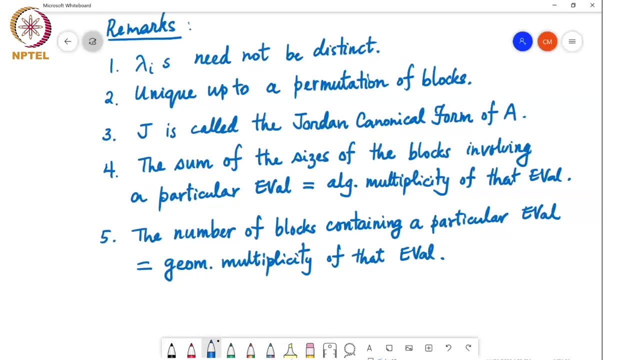 value. it means that all the Jordan blocks will be of size 1 cross 1.. And for every Jordan block you will have one linearly independent Eigen value, Eigen vector. So this point is a little. It is something good to know, but I will not elaborate on it because it requires me to. 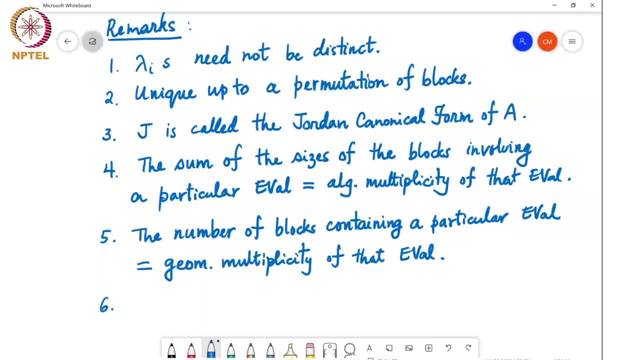 explain about the concept of, Of minimal polynomials, which I will come to a bit later, But for now I will just make a note here. Maybe we will go back and look at this when we discuss minimal polynomials. So the largest block involving a particular Eigen value. 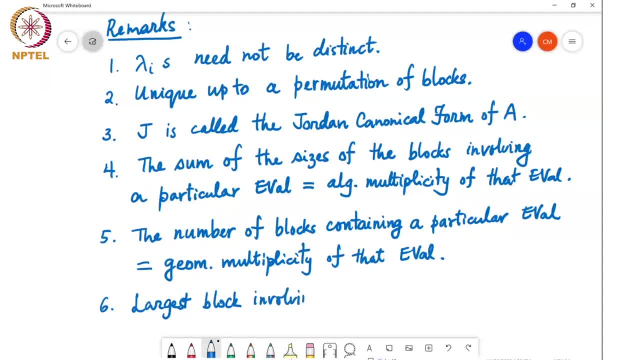 So the largest block involving a particular Eigen value. So the largest block involving a particular Eigen value Is the multiplicity of? Is the multiplicity of? Is the multiplicity of That Eigen value in the minimal polynomial of A, That Eigen value in the minimal polynomial of A? 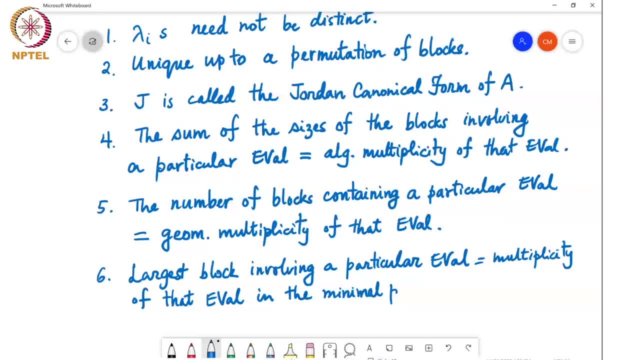 That Eigen value in the minimal polynomial of A. So basically, this minimal polynomial of A is essentially So for now, just for the sake of completeness, I will write this here. So the minimal polynomial Is, Is, Is. 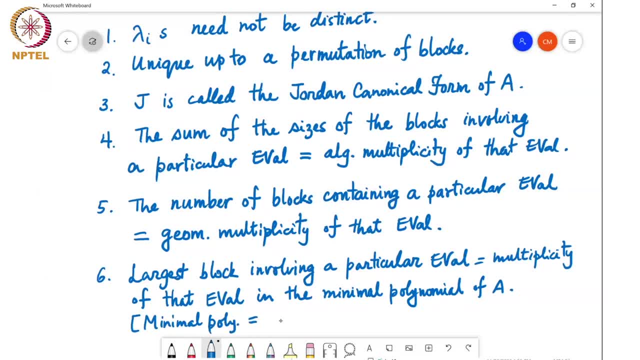 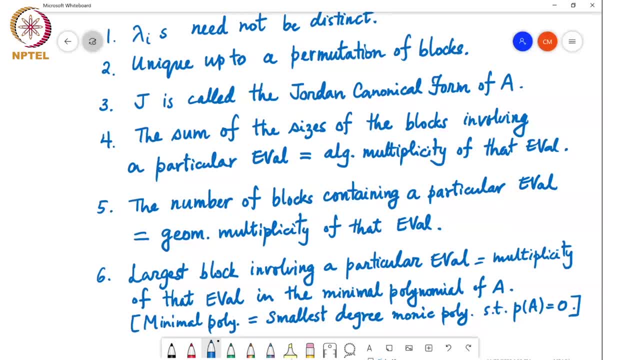 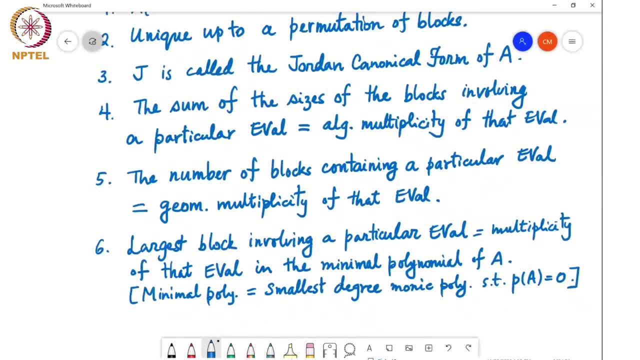 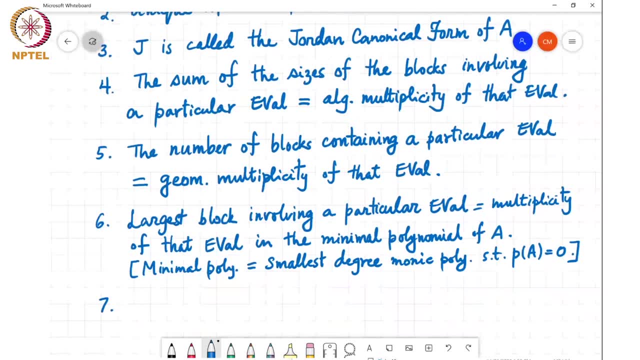 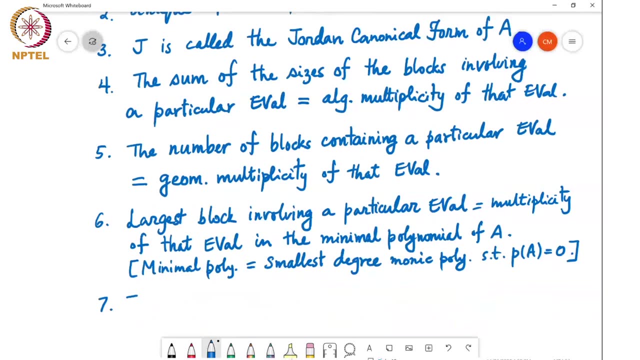 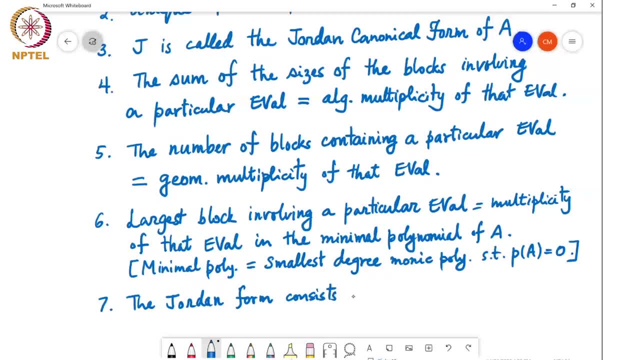 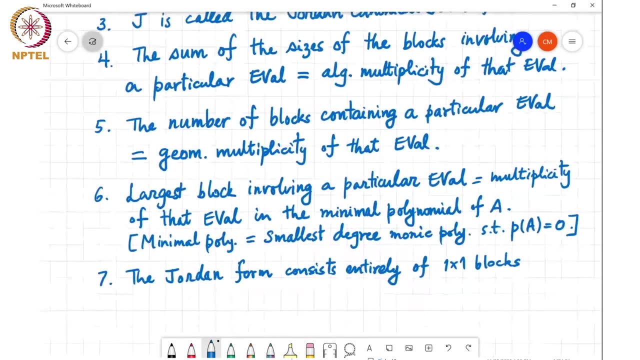 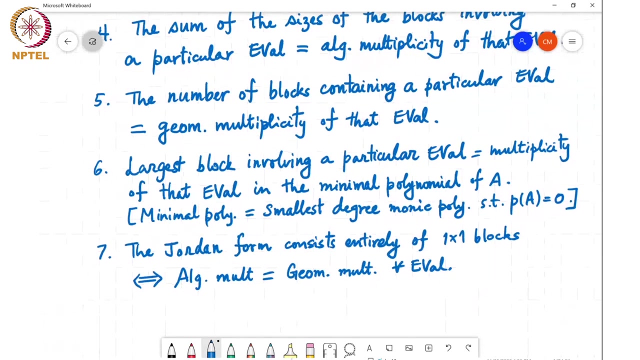 then basically there are no super diagonal elements in the Jordan canonical form of the matrix and that implies that the algebraic multiplicity equals the geometric multiplicity for every eigenvalue and the Jordan form is actually a diagonal matrix. You can imagine that for a, you can easily see that for a matrix that is diagonalizable, the 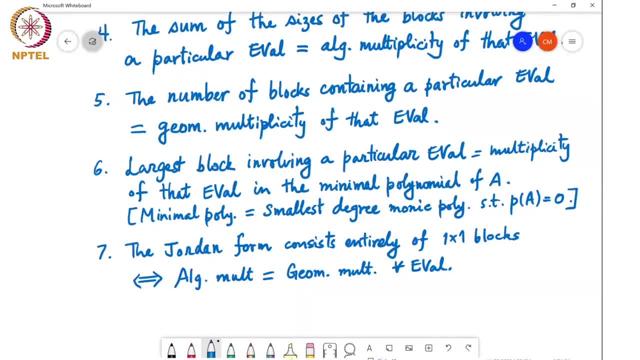 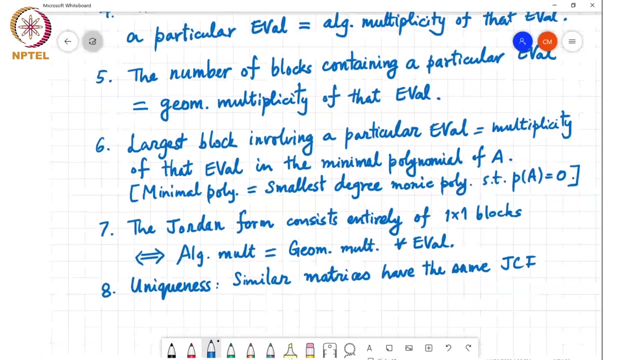 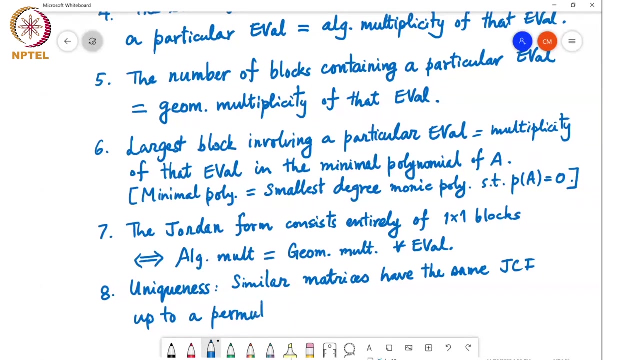 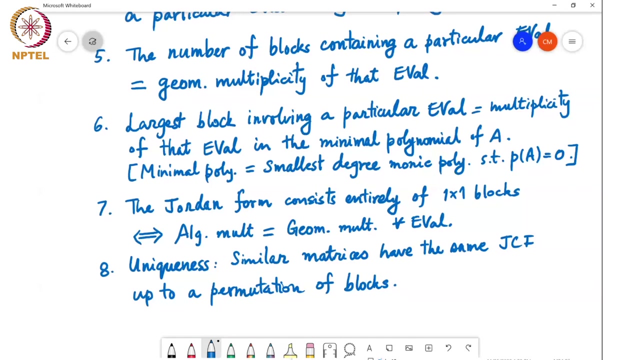 Jordan canonical form will come out to be a diagonal matrix. So uniqueness: similar matrices will have the same Jordan form, up to a permutation of blocks, For example the. So let us maybe look at one or two examples and see how this looks like. 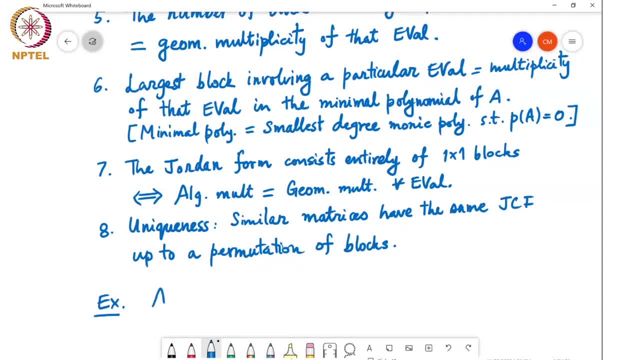 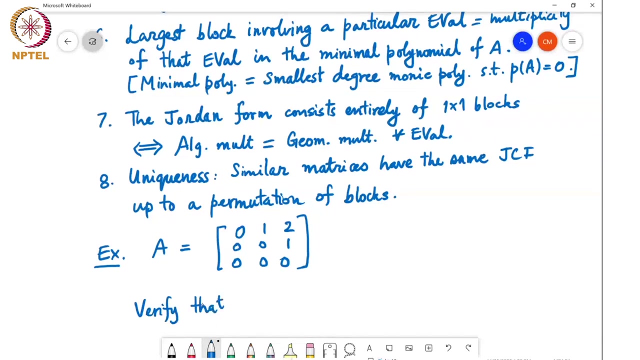 So if I take, for example, A equals the matrix 0, 1, 2, 0, 0, 1, 0, 0, 0.. Okay, then one can check that If I do. 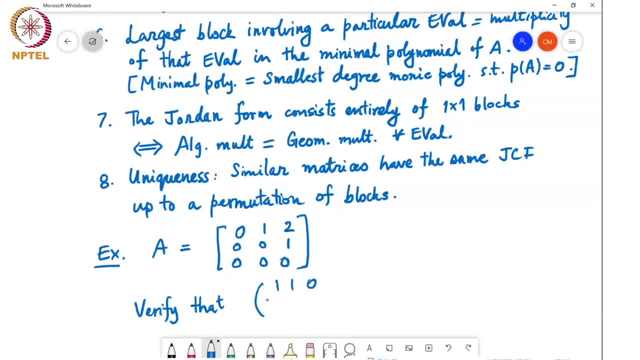 1 1 0 0, 1 2 0 0. 1. inverse times: 0 1 0 0 0. 1 0 0 0. times: 1 1 0 0, 1 2 0 0. 1.. If I carry out this: 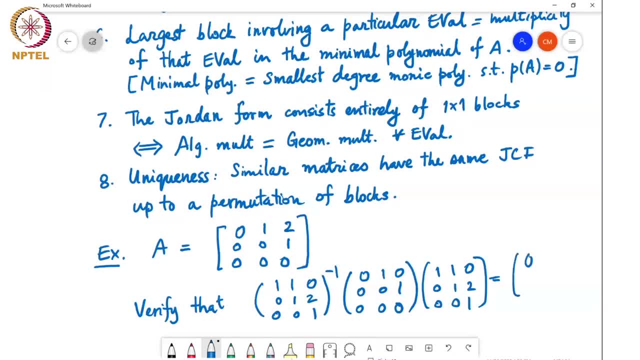 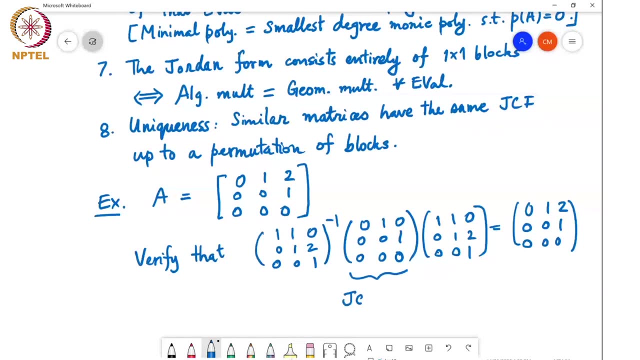 multiplication, I will get this matrix: 0, 1, 2, 0, 0, 1 and 0 0 0.. So basically, this matrix in between here this is the Jordan canonical form, which is actually equal to J 3.. It is a. 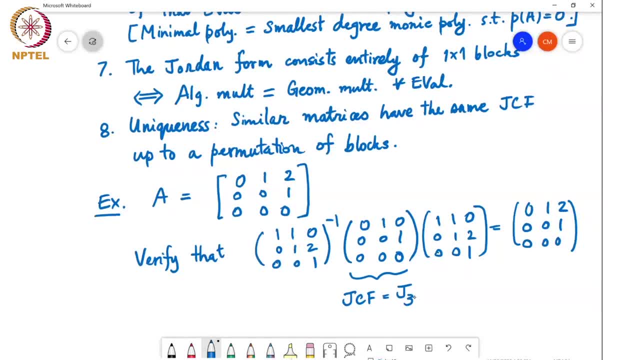 3 cross 3 matrix here. So it is again a notational abuse here, because I had written J 1,, J 2, etc. where J i was an n i cross, n i block. But nonetheless I will write it like this: 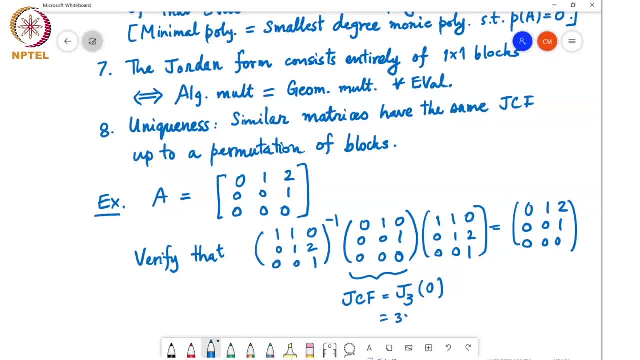 It is a 3 cross, 3 block, Jordan block, with lambda equals 0.. See, this is an upper triangular matrix. Its eigenvalues are all equal to 0.. That is obvious, But this is the simplest form You can reduce the matrix. 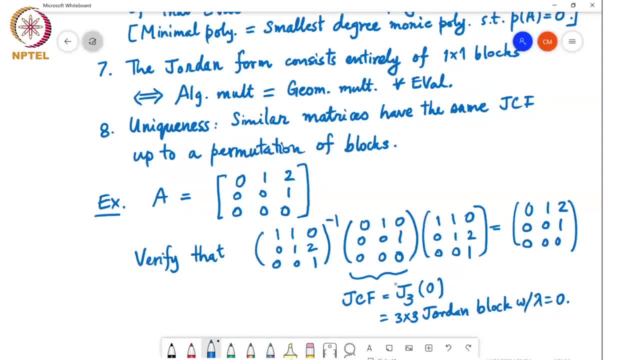 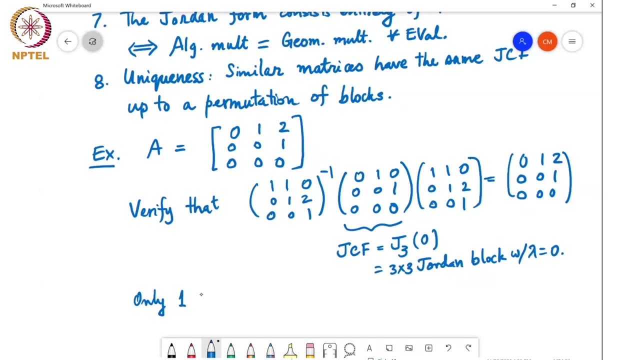 And this is the matrix 2, which is a Jordan block of size 3, cross 3, associated with eigenvalue 0. So, basically, this matrix has only one eigenvalue, one distinct eigenvalue- lambda equals 0. So this lambda equals 0 has algebraic multiplicity 3,. 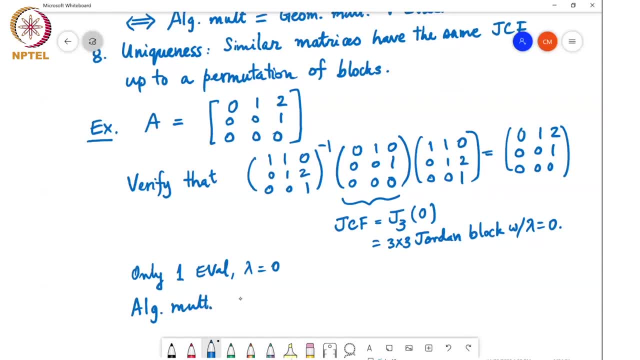 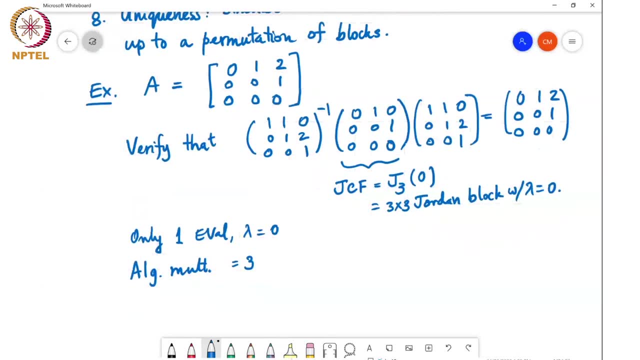 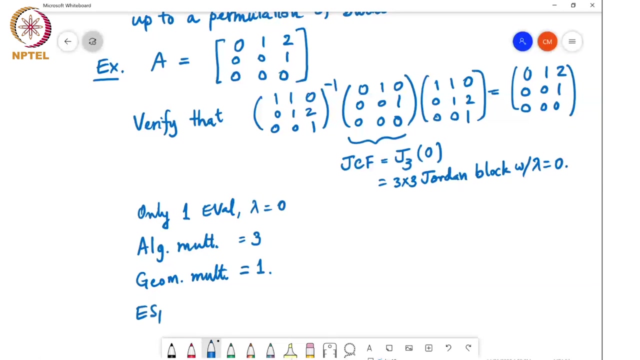 and geometric multiplicity equal to 1.. The eigenvalue 0 occurs in only one block of size: 3, cross 3.. So basically, if I asked what is the eigenspace of lambda? equal to 0. the set of vectors: alpha: 1: 0, 0. 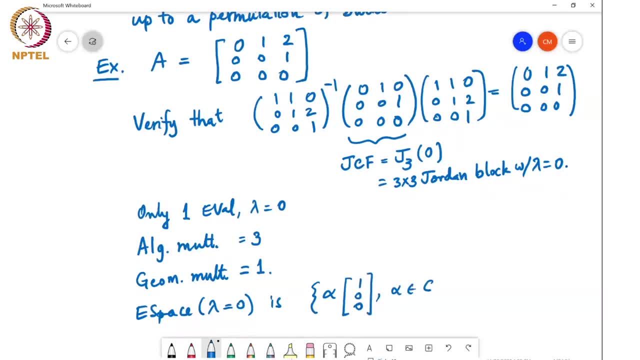 alpha and c. So I take any vector like this and multiply it with this matrix, I will get 0 times this vector: 1 0, 0.. So it has only one linearly independent eigenvector corresponding to lambda equals 0. So it is a defective matrix. 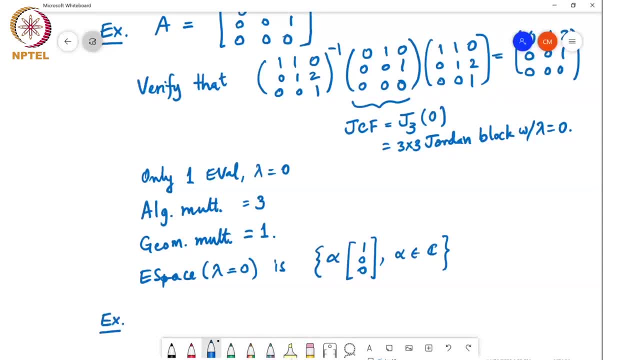 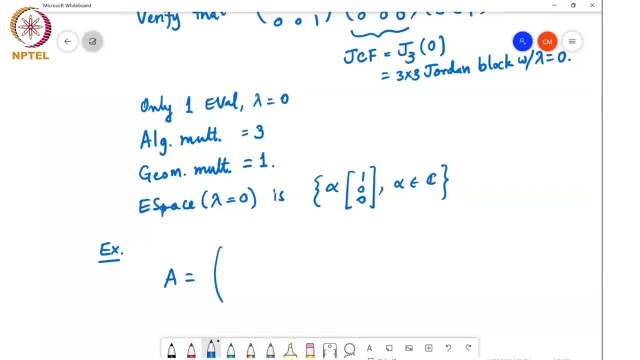 So here is another example. Now we take a slightly more elaborate example. So minus 2 minus 1 minus 3.. 4, 3, 3 minus 2, 1 minus 1.. If I asked, what is the characteristic polynomial of this matrix? 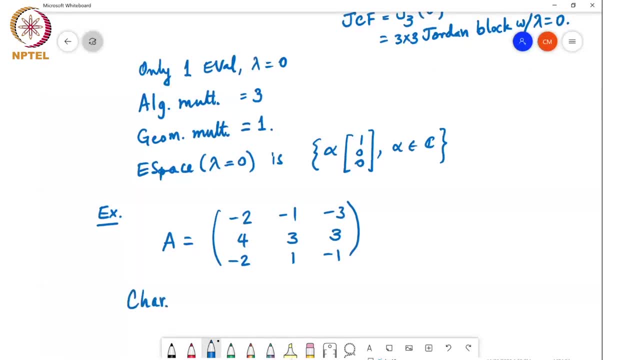 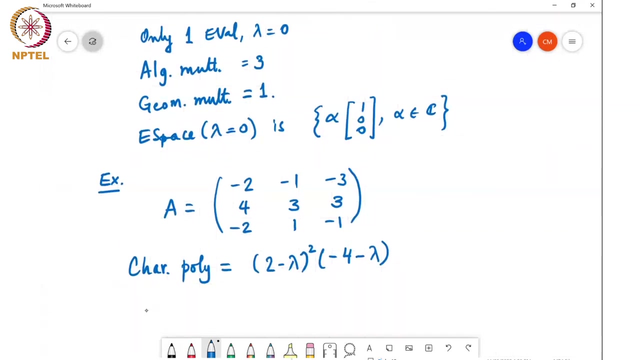 you can work it out. So it simplifies to 2 minus lambda the whole square Times minus 4 minus lambda, And so that implies that the eigenvalues are 4 and minus 2.. Minus 4 and 2. And these have. 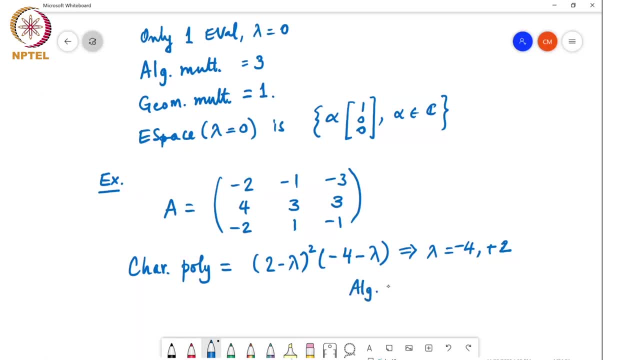 algebraic values. So this is the algebraic multiplicity. So, corresponding to minus 4, the algebraic multiplicity is 1.. Corresponding to 2, the algebraic multiplicity is 2.. So 2 occurs twice as the solution to the characteristic polynomial. 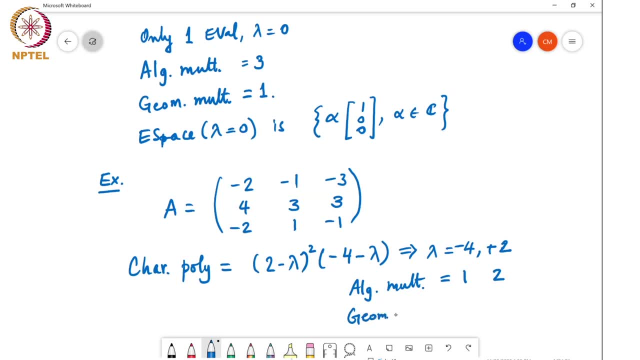 And the geometric multiplicity is at most the algebraic multiplicity, And in this case it turns out to be 1 and 1.. It is always equal to at least 1. And it is at most equal to the algebraic multiplicity. 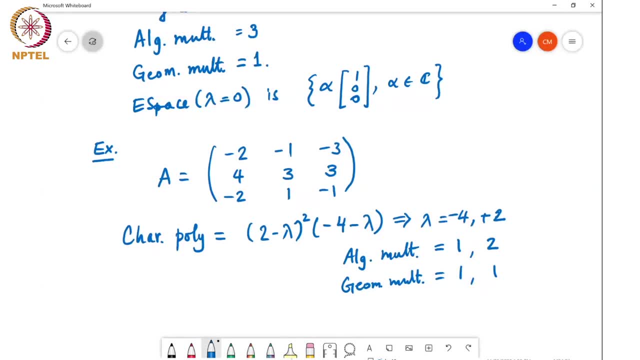 So these things you take on faith for now. We will actually see how to compute the Jordan canonical form next, And then you will be able to execute that for this matrix And see that all these are true. So the Jordan canonical form for this matrix is: 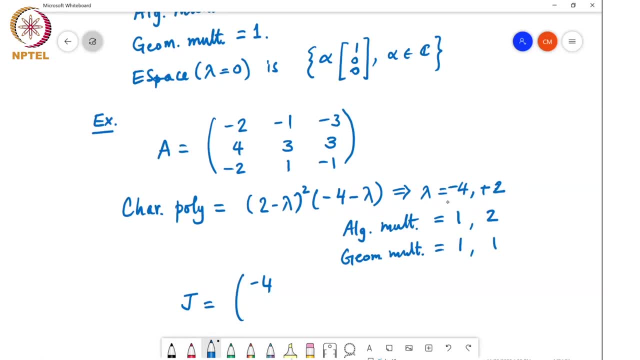 minus 4.. So there will be two blocks. One block will correspond to the eigenvalue minus 4.. And since the other one has a geometric multiplicity of 1 and an algebraic multiplicity of 2.. The other block is a 2 cross 2 block with eigenvalue equal to 2..